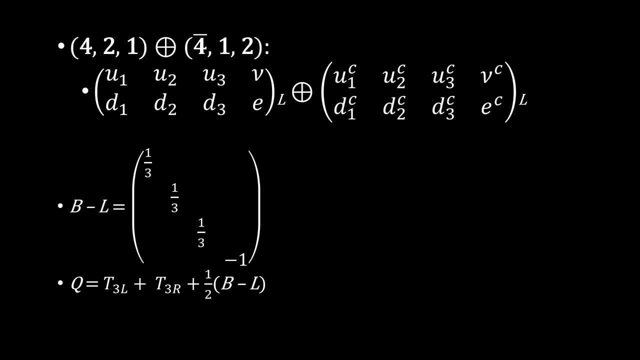 We conjugated the right-handed fields to write all whale fields as left-handed fields For the Perti-Solom theory. it is convenient to undo this At the cost of introducing unobserved right-handed gauge bosons. we have made the world more. 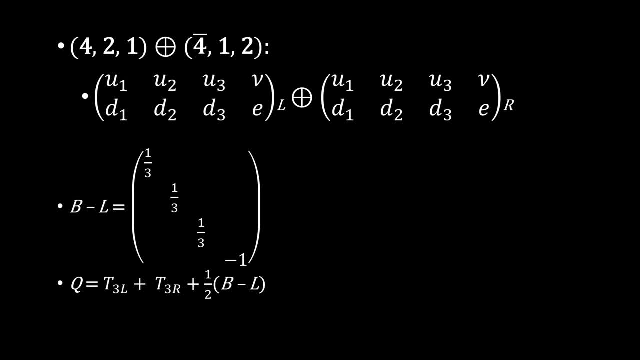 practical, We are forced to introduce a field nu R with the quantum numbers of the right-handed neutrino and to explain the fact that no such particle is observed experimentally by giving it a very large Majorana mass. This model explains charge quantization, while electric charges are integer multiples of 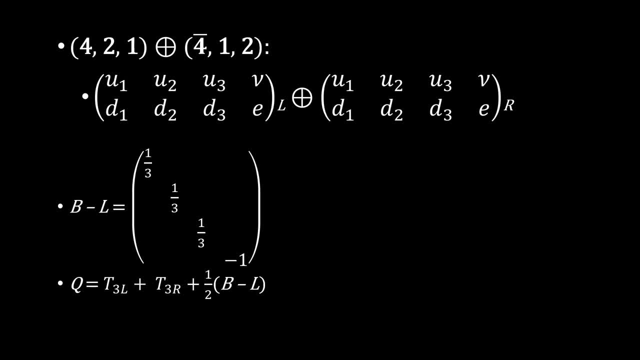 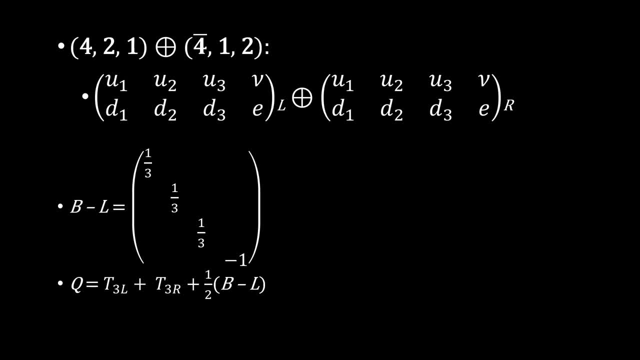 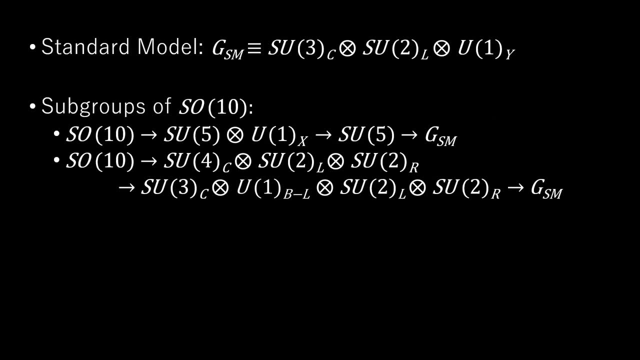 The Perti-Solom is a very important element in the Perti-Solom model. Incorporation of the diagonal generator implies that quarks charges are expressed in terms of one-third fractions of leptons charges, SO has two inequivalent maximal subgroups and hence breaking patterns. SO goes to su5. 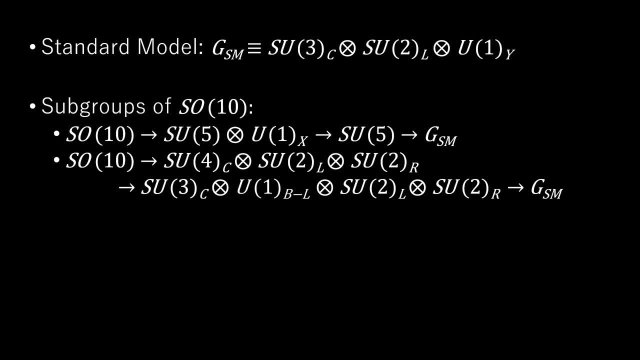 cross u1 x and SO goes to su4. cross su2 L, cross su2 R. Gauge coupling unification remains intact. in the case for the breaking pattern, SO goes to su5.. For intermediate dissection, CO locals disappeared from U2 and L to U2..